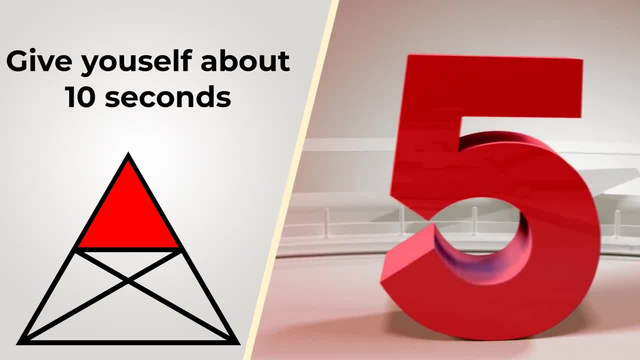 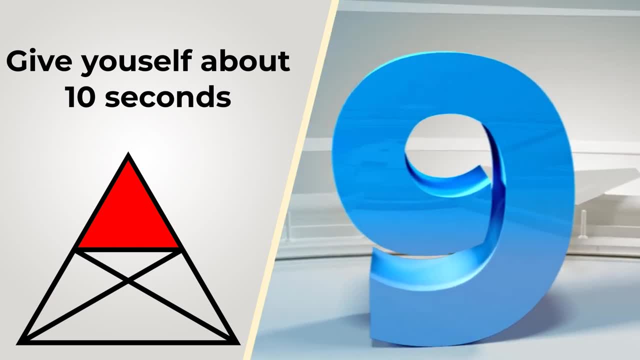 Give yourself a few seconds. I would recommend 10 to 15 seconds. This is about as much time as you will get in the real test. You can pause this video to give yourself some time to figure out the answer. I'm going to continue and reveal the correct solution. 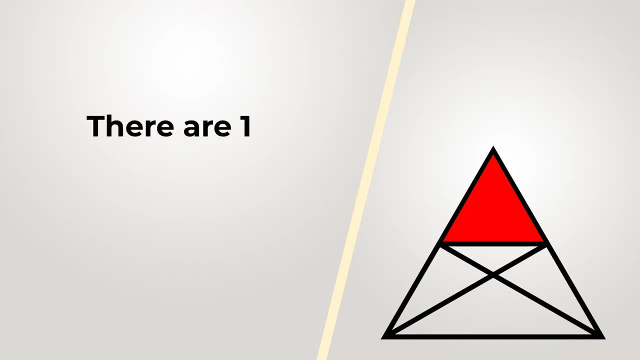 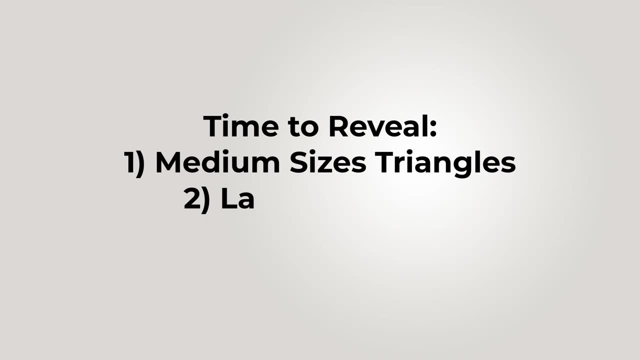 so we can get to the answer together. I counted 12 triangles in this picture. Is this what you got too? Let me show them all for you. I'll start with the smaller triangles and then go to the medium-sized ones and then go to the large ones. 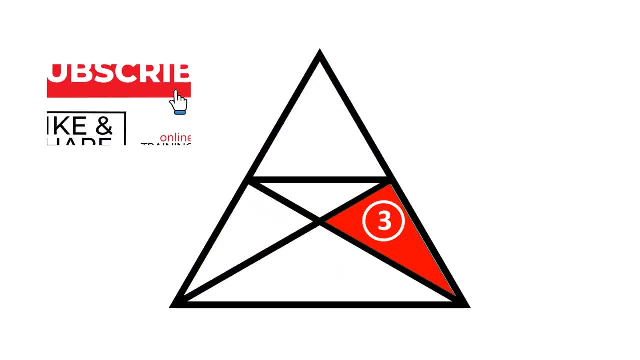 One, two, three, four, five, six, seven, eight, nine, ten. One, two, three, four, five, six, seven, eight, nine, ten, eleven and twelve. Did you come up with the different answer? 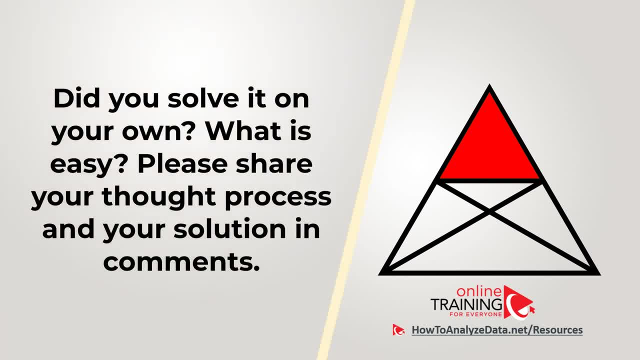 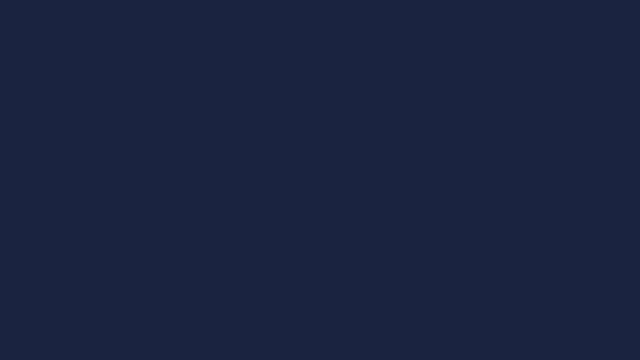 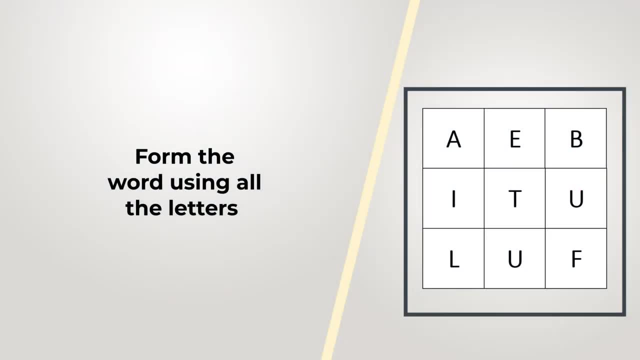 Please share your thought process in the comment section of this video so we can all learn from your perspective. Hopefully you nailed this question and got to the correct answer on your own. Here is the tricky question which tests your imagination, knowledge of English words and logical reasoning. 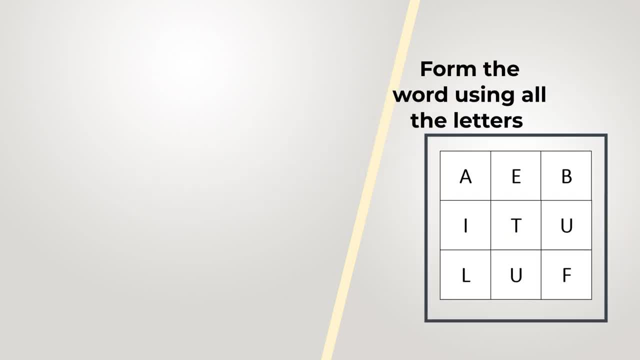 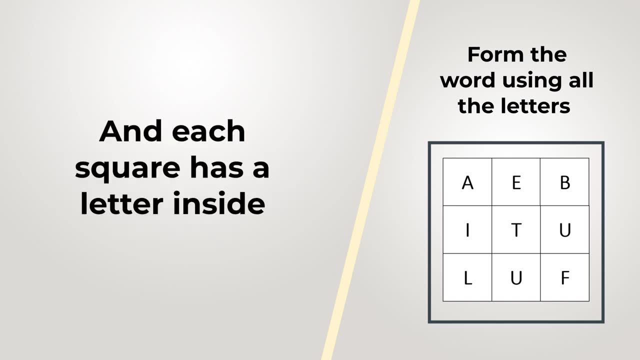 What word can you form using all the letters in the box? And you're presented with the box that contains nine squares and each square has a letter inside. Take a closer look at this picture and see if you can come up with the answer. This might be the right time to pause this video. 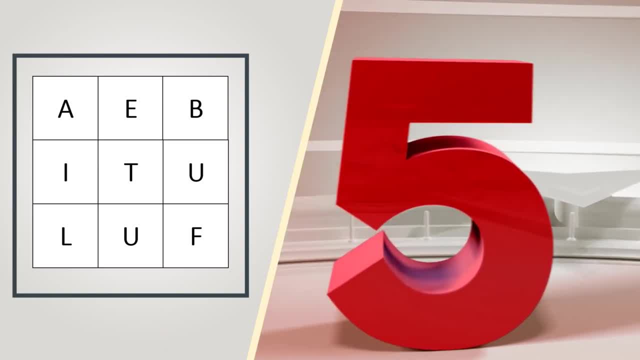 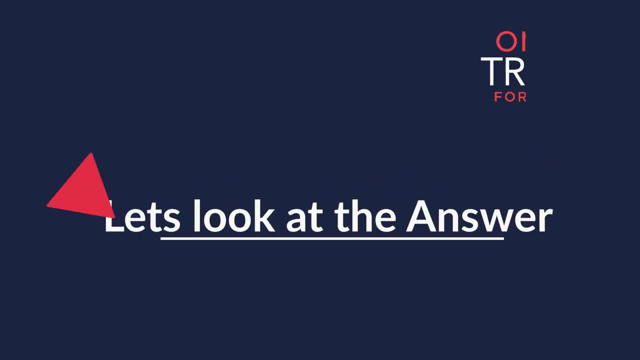 to see if you can come up with the answer on your own. Do you think you know the answer? Let's continue to see how we can solve this and get to the correct solution together. Obviously, there are quite a few words that can be formed with these letters. 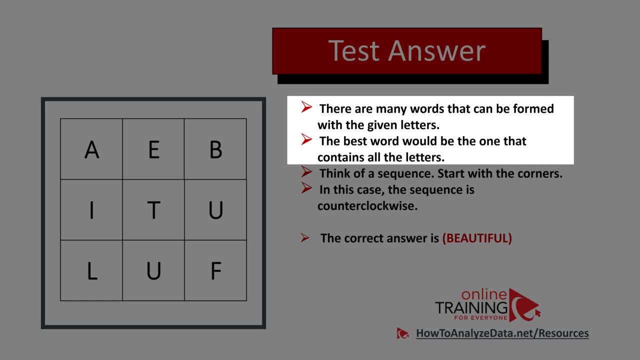 But the best word will only contain one of each of the nine letters presented here on the screen. The best solution here is think of the sequence. A lot of times authors of this question put letters in the opposite orders of the way we currently read this. 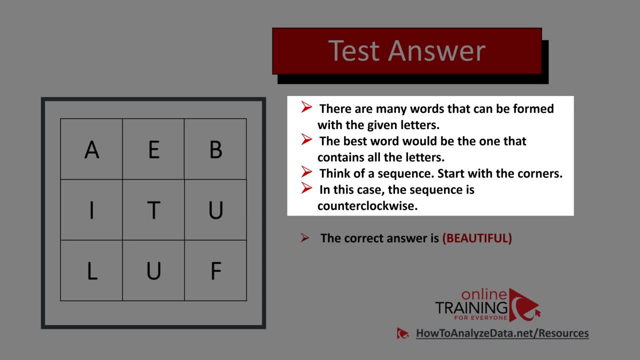 So, for example, if we read left to right or top to bottom, they might put word letters that will go in the sequence from right to left or from bottom to the top, And this is exactly the case here. The correct answer here is word beautiful. 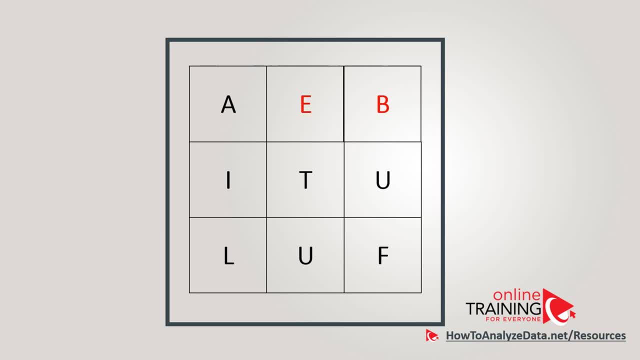 which starts in the upper right corner, And then you go by the letters B, E, A, U, T, I, F, U, L, And that's how you get to the correct answer, which is the word beautiful. Hopefully you've nailed this question and now know how to answer similar problems on the test. 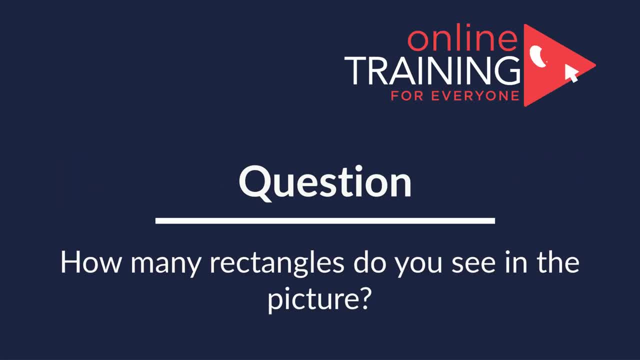 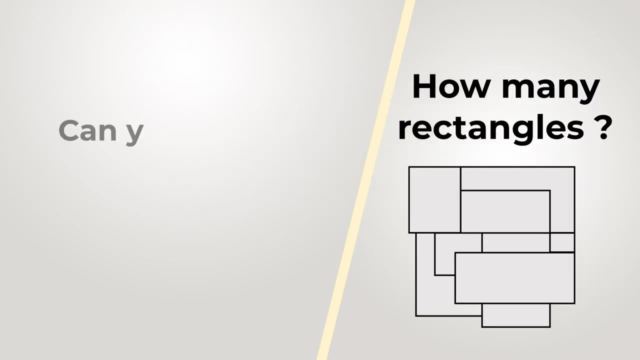 I'm very excited to share with you the problem that tests your analytical skills, And there is a very high chance that you will see it on the test. How many rectangles do you see in the picture? You are presented with the shape on the left. 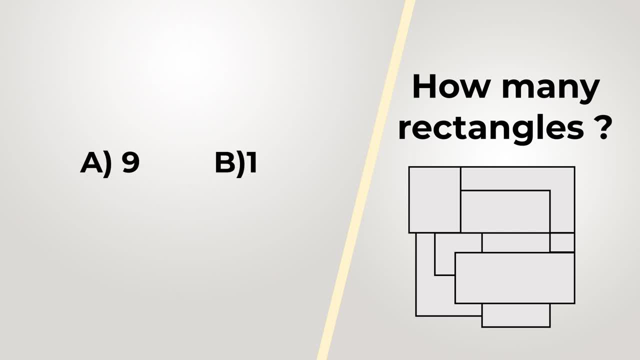 and four different choices: Choice A- 9,, choice B- 12,, choice C- 17, and choice D: 24.. Take a close look at the picture and then take 10 to 15 second break to see if you can count all the rectangles. 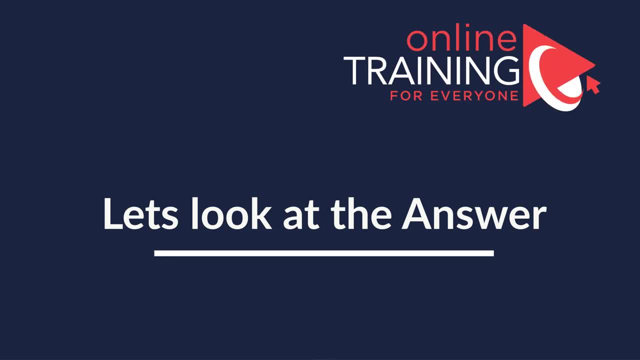 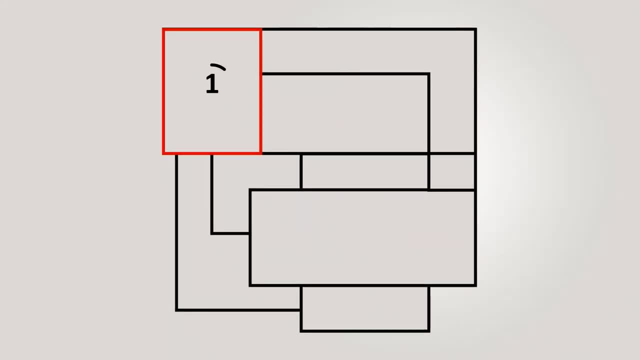 Let's look at the solution together to see if we've got it right. There are nine rectangles you can see on this picture. Let's count them all together: One, two, three, four, five, six, seven, eight and nine. 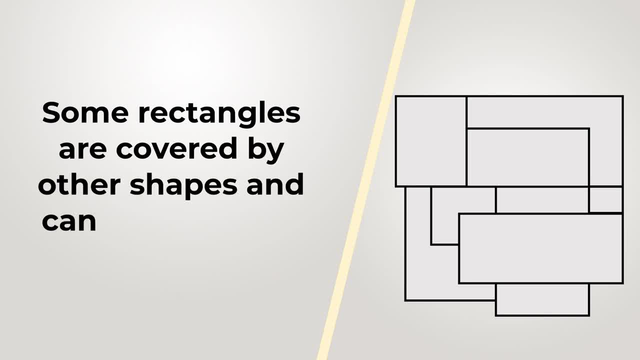 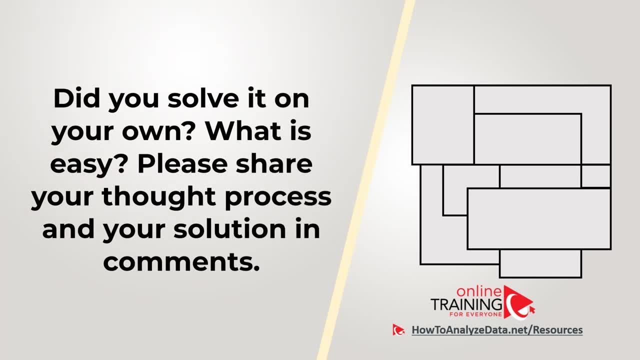 Some rectangles are covered by other shapes and cannot be counted. How did you solve it? Did you come up with a different answer? What was your thought process? Please share in the comments section of this video so we can all learn from it. Hopefully you've nailed this question. 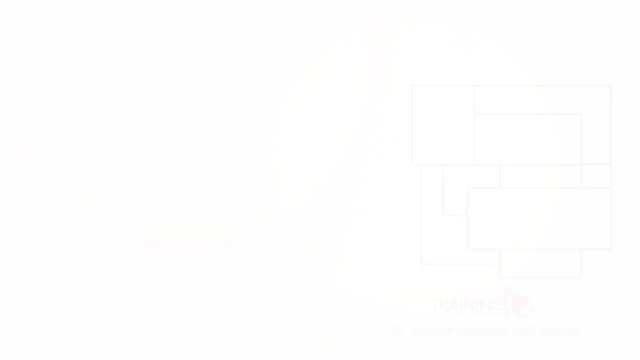 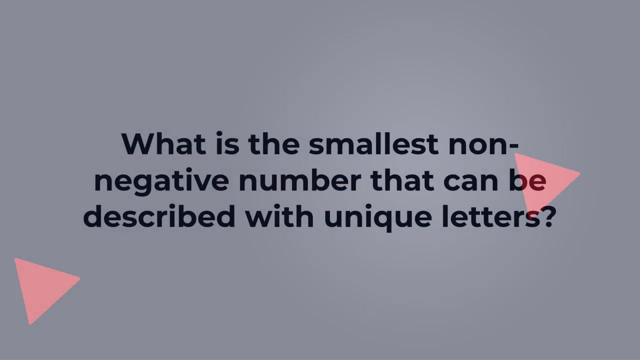 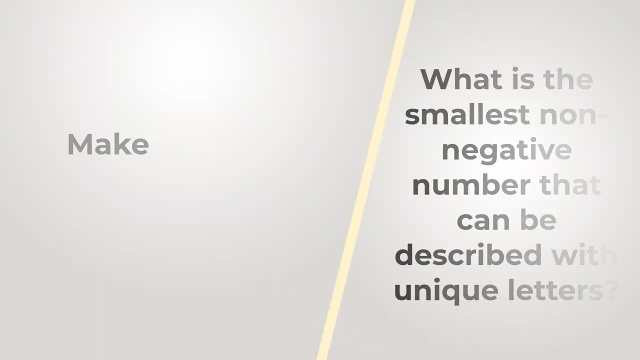 and now know how to answer similar problems on the test. Here's the challenging question you might frequently see on the test: What is the smallest non-negative number that can be described with unique letters? You might have to re-read this question multiple times just to understand what is being asked. 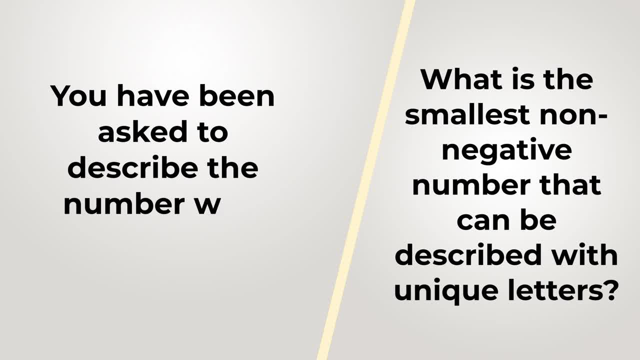 Let me help you If we are to clarify this question. you are being asked to describe the number with the letters, And those letters should be unique. For example, in word 20, there are two letters, T, So 20 is not the word that can be used in the test. 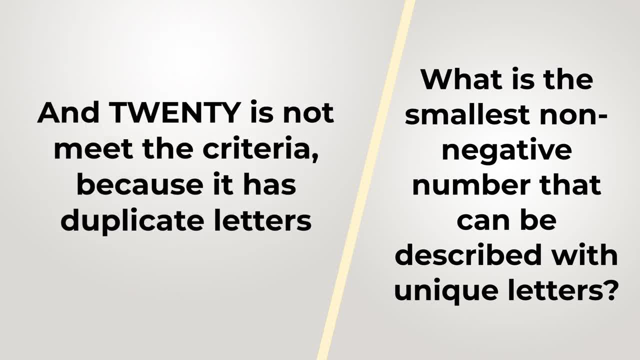 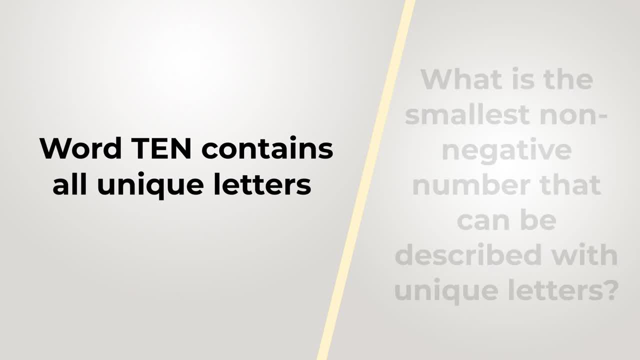 On the other hand, so, which means that 20 is not the word that meets the criteria because it has duplicate letters. On the other hand, word 10 contains all unique letters. So the question is: what is the smallest non-negative number that can be used in the test? 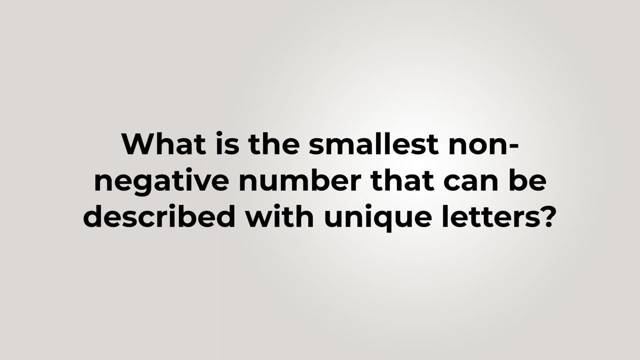 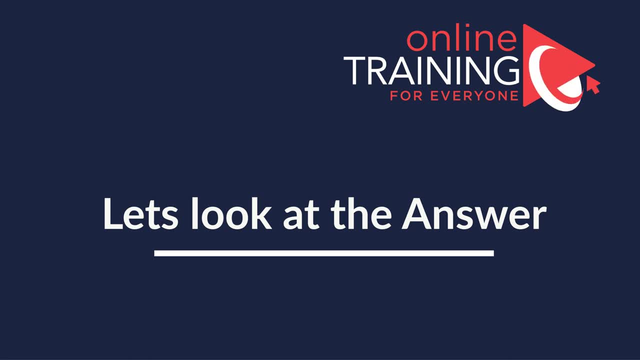 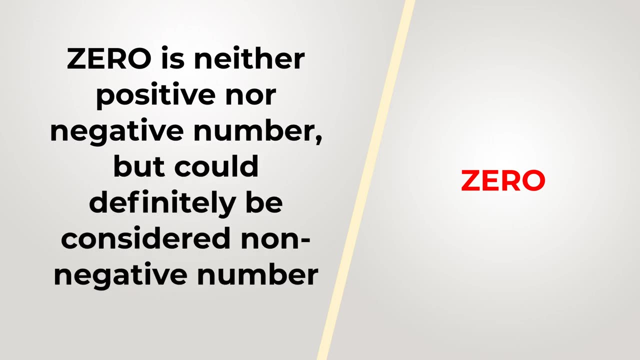 What is the smallest non-negative number that can be described with unique letters? A lot of times people get the answer 1, and this might be true because 1 is the positive and all letters are unique, But the actual answer to this question is 0. 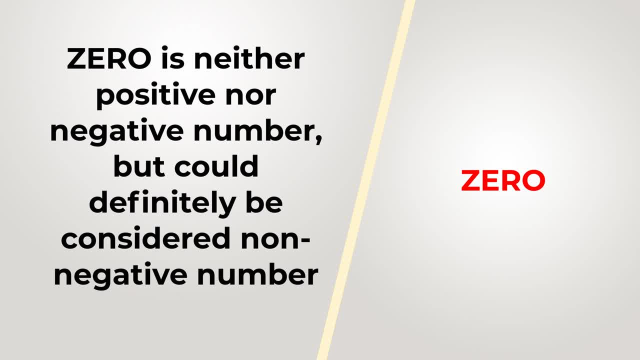 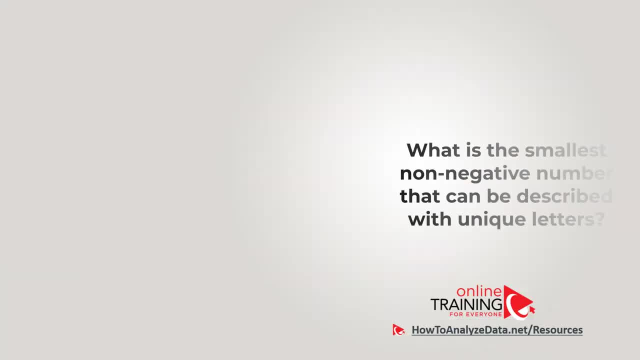 because 0 is neither positive nor negative number, but can definitely be considered as a non-negative number. So the correct answer here is 0.. Did you figure it out? Please share your thoughts and the way you approach this question in the comment section of this video. 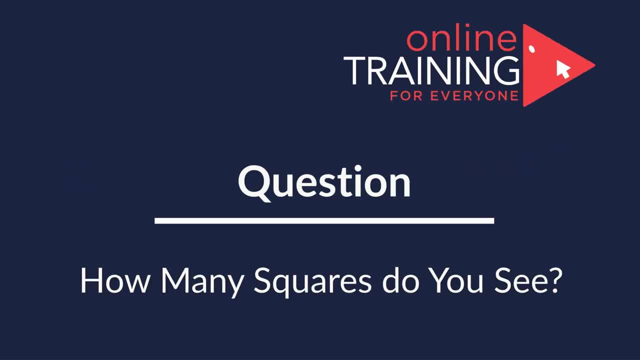 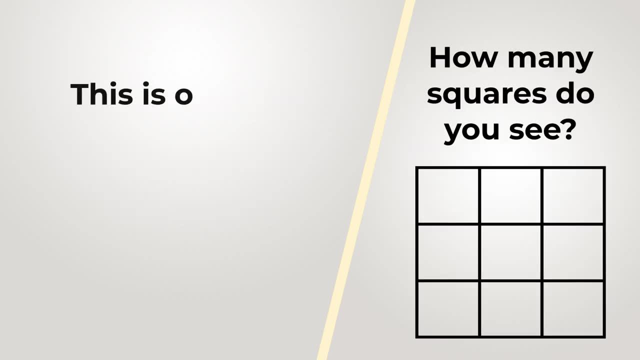 I'm very excited to share with you this question, which we frequently see on the test. Despite being tricky, you will have a lot of fun trying to find the answer. This is one of those questions that is easy to understand and it challenges your brain and improves your IQ. 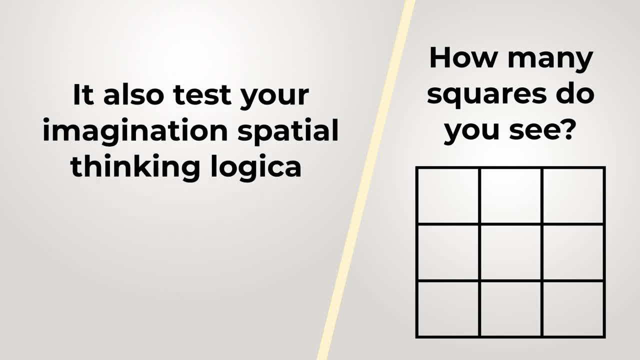 It also tests your imagination, spatial thinking, logical thinking and attention to details. Take a look at the picture and see how it works And if you have any questions, feel free to ask them in the comments section of this video. And if you have any questions, feel free to ask them in the comments section of this video. 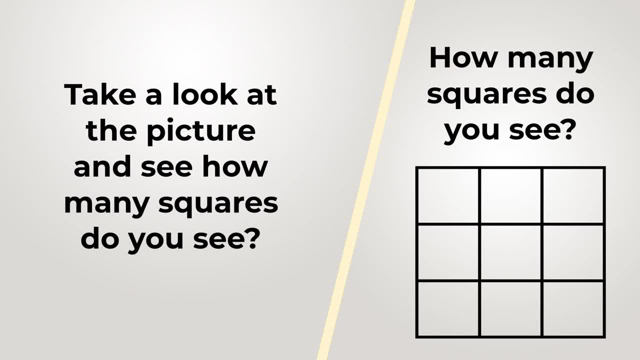 How many squares do you see? Think again. The answer might be more challenging than you think. Now might be the good time to pause this video to see if you can come up with the answer on your own. Give yourself about 10 seconds. 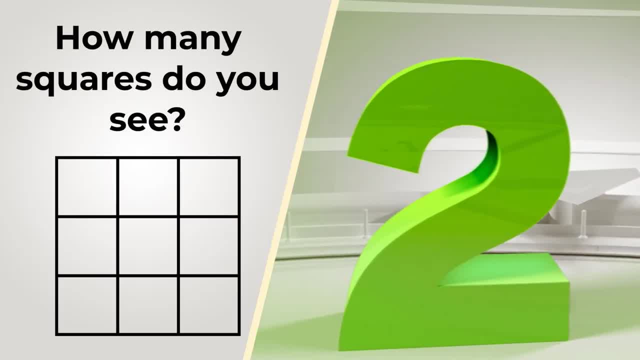 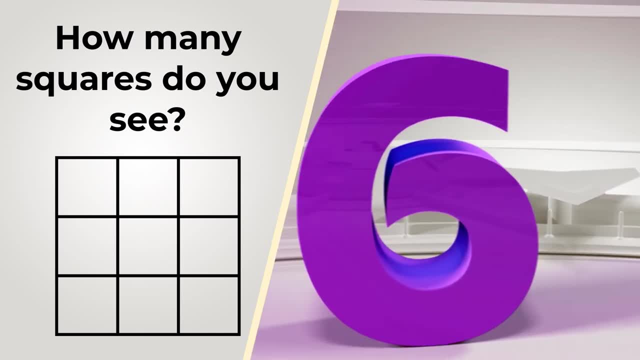 This is typically how much you will get on a real test. Do you know the answer? Let me give you a tip. Keep in mind, though, that on a real test, most of the time you don't get any tips, But since we are doing it together, 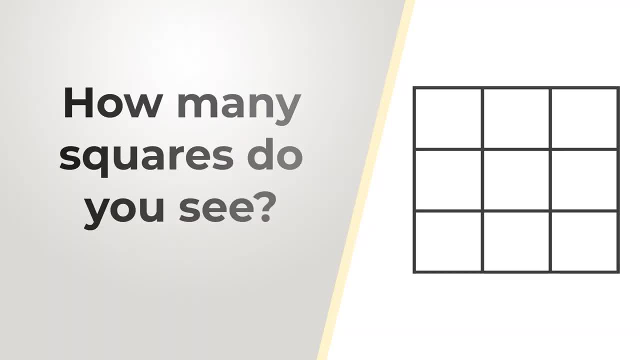 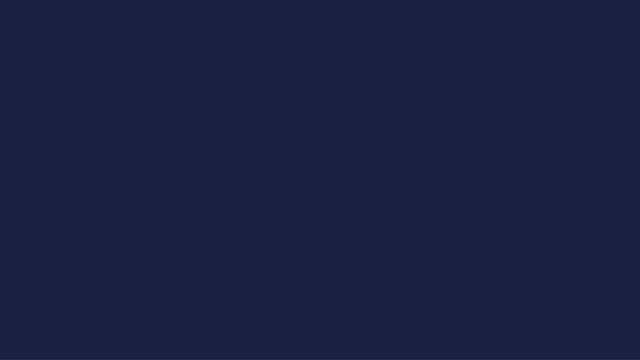 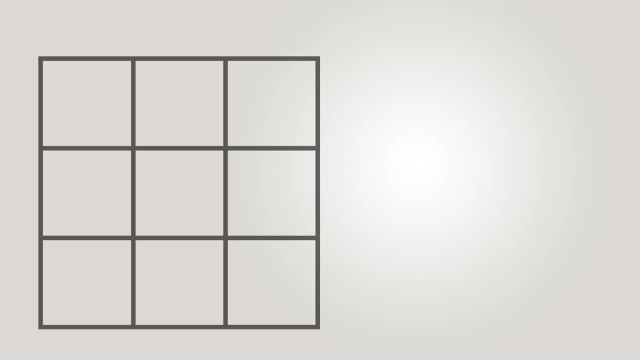 I'd like you to consider the possibility of one shape being inside the other. Let's continue to see how we can solve this challenge and get to the correct solution together. There are 14 squares that can be identified in this picture. This definitely came as a big surprise to me. 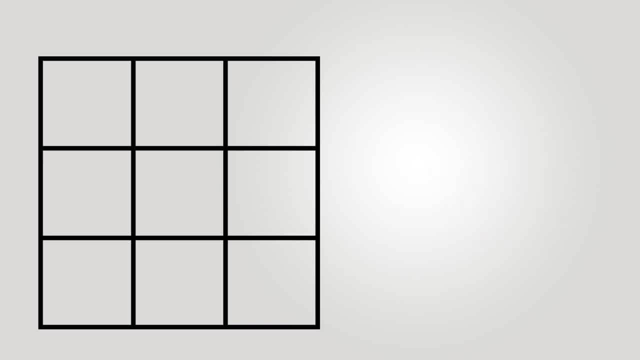 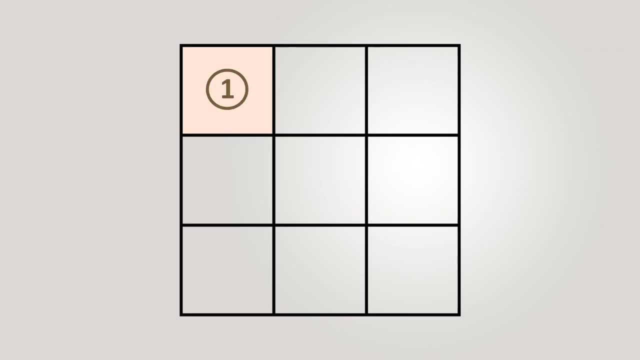 Do you see them all? Some of them might be much easier to identify than others. Let me draw them for you. There are 9 small squares: 1,, 2,, 3,, 4,, 5,, 6,, 7,, 8, and 9.. 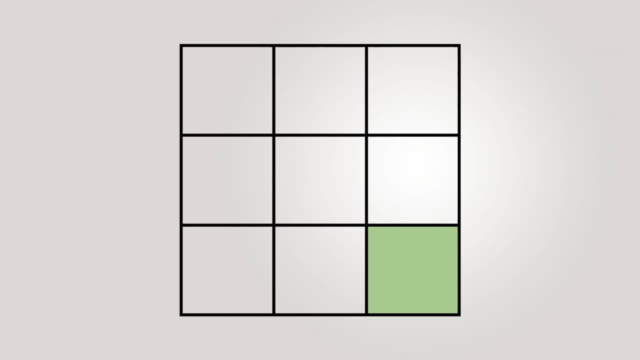 Even those small squares are easy to see and identify. Let's look at the medium-sized squares. There are 4 of them: Number 10., Number 11., Number 12. And number 13.. And then there is one large square. 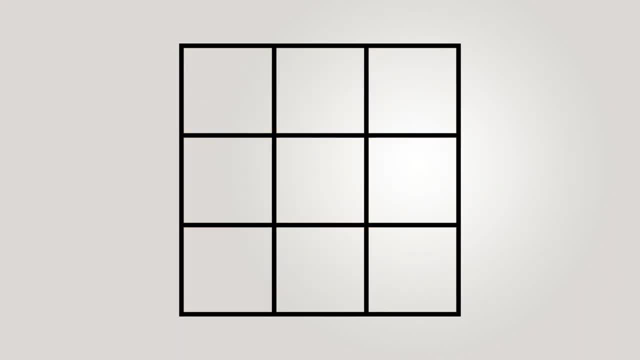 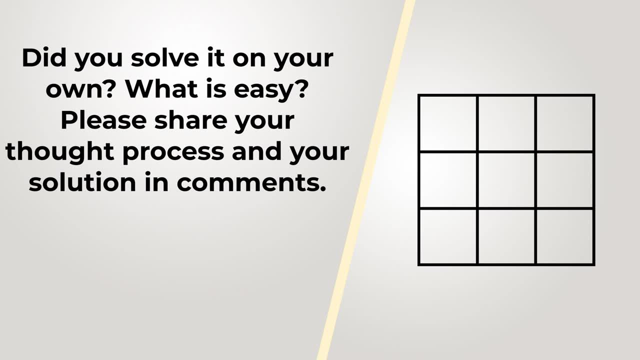 This is number 14.. What do you think about this challenge? Were you able to solve it right away? In case you see some additional shapes that we missed, which is always a possibility, please make sure to share them in the comments of this video. 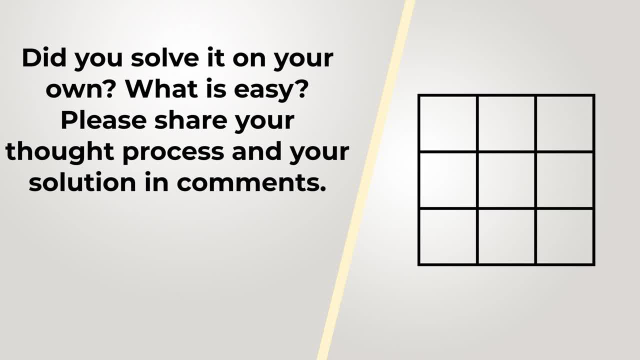 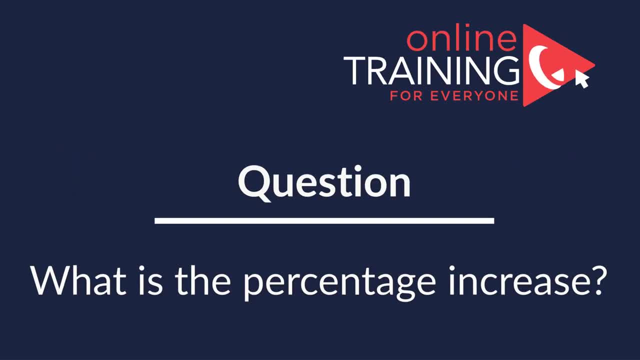 Hopefully you've nailed this question and now know how to answer similar problems on the test. Thank you for watching. Don't forget to like and subscribe to our channel. See you in the next video. Bye-bye. Here is a frequent question on the test that a lot of people get wrong. 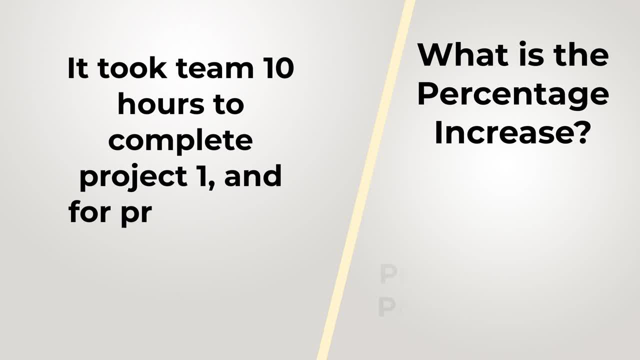 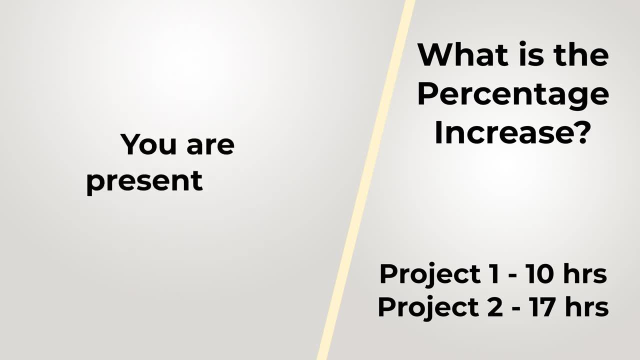 It took 10 hours to complete project 1.. For project 2, it took 17 hours. What is the percentage increase between two projects? You are presented with 4 different choices: Choice A – 7%. Choice B – 17%. 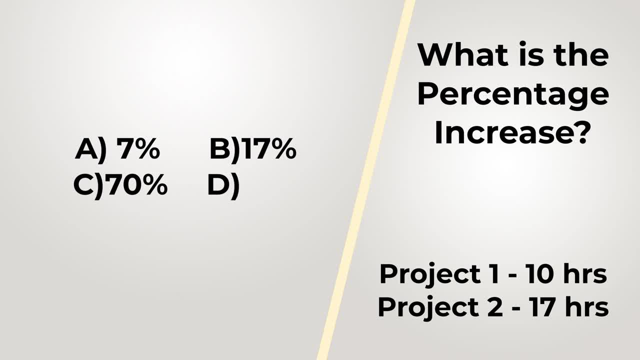 Choice C – 70% and then Choice D – 170%. Take a close look to see if you can calculate and come up with the right answer. You can pause this video and give yourself a little bit of time to better understand what is being asked. 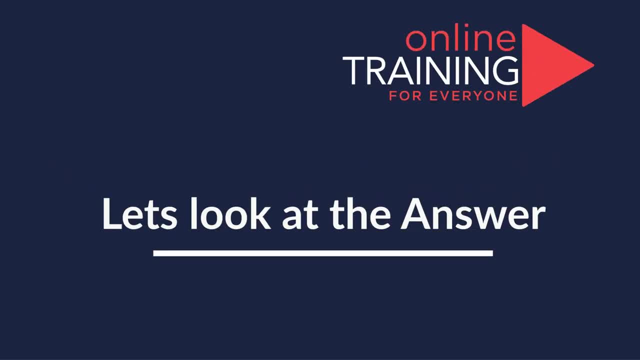 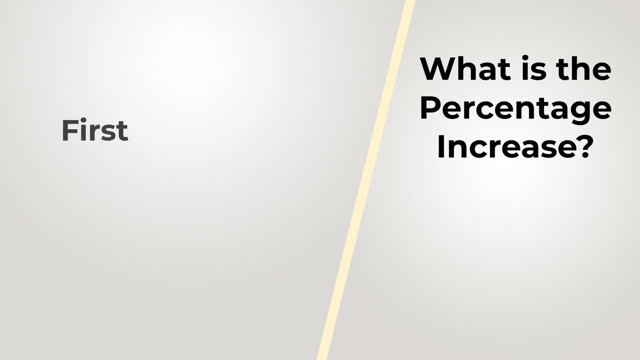 Do you think you know the answer? Let's continue to see how we can figure out and get to the correct solution together. To calculate percentage increase, you need to do the calculations First. you need to determine the increase in hours. To do that, you need to subtract project 2 hours from project 1 hours. 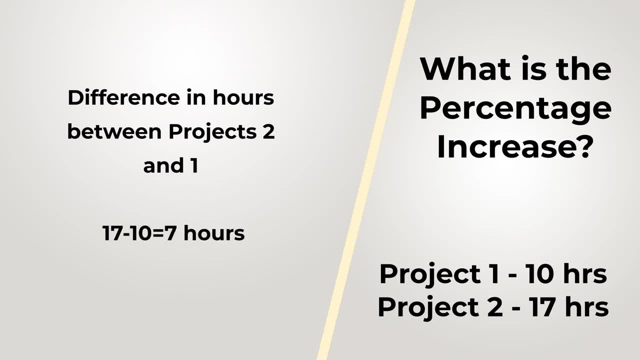 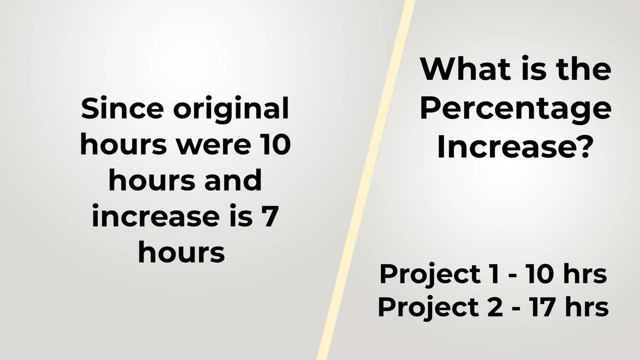 To do this, you need to do 17% minus 10 and the result would be equal to 7 hours. This represents the increase in hours between two projects. In the next step, you need to divide the increase by original hours, Since original hours were 10 hours and increase is 7 hours. 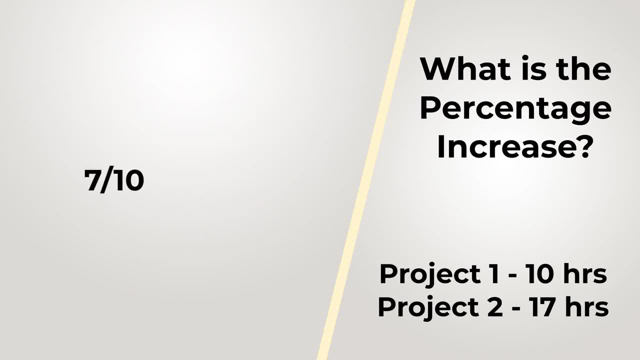 what you need to do? you need to divide 7 by 10.. And, as a last step, you need to multiply it by 100%. You can do the calculations in your head or if you use a calculator, you will come up with the same result, which will be 7.. 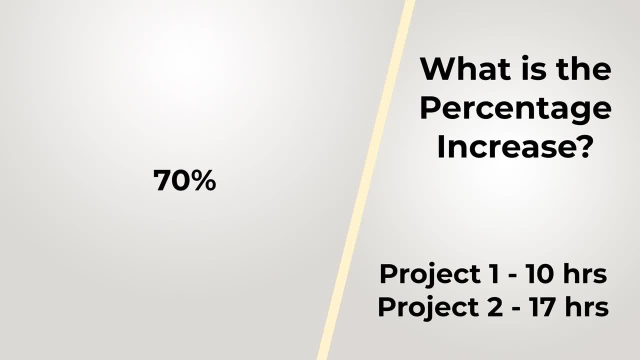 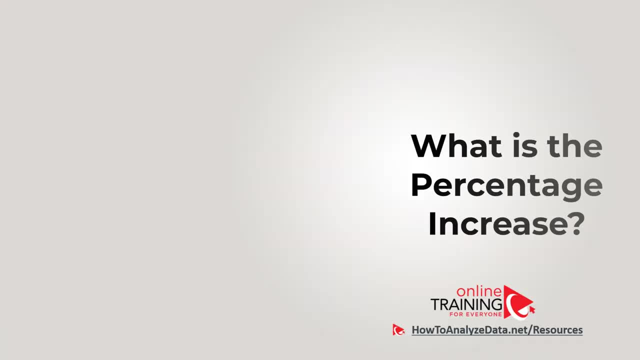 So the correct answer here is the increase was 70% and the correct choice here is C. Did you figure out the correct answer? Please share your thought process in the comments section of this video so we all can learn And, if you need more similar problems, to practice for aptitude tests. 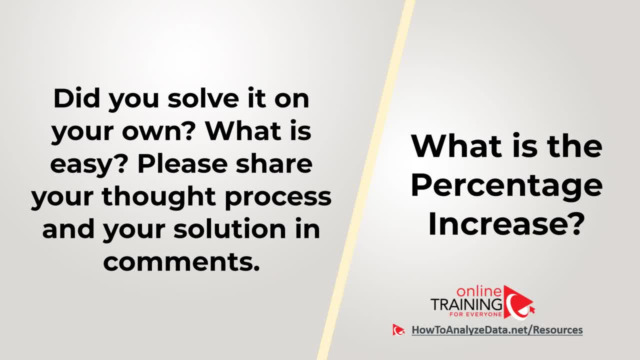 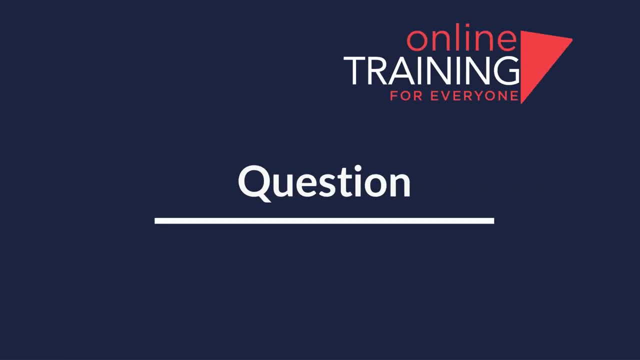 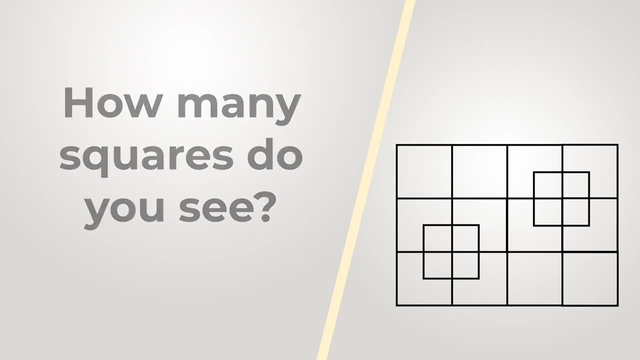 please make sure to check out my ebook in the comments section of this video. I gotta tell you I love the fact that you are using a calculator And I am sure that you will also like it. you. i love this question. this is such a unique question and we see a lot of variations of this. 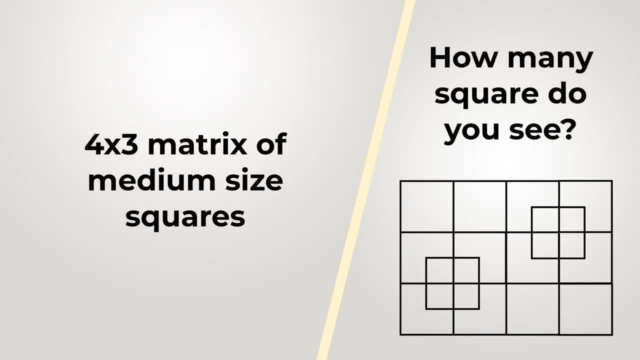 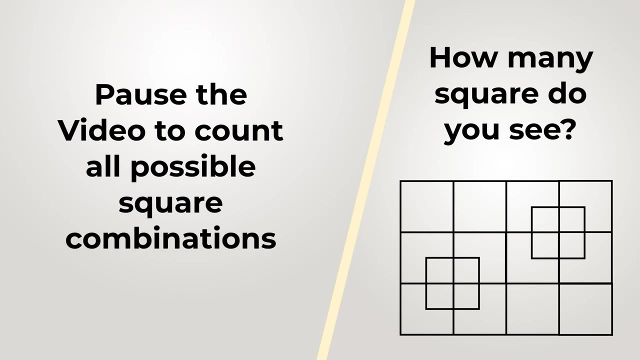 question. in the test, in this particular version, you are presented with the 4x3 matrix of squares and then you see two additional squares on top of the medium-sized squares, and the question is: how many squares do you see on the picture? take a closer look and give yourself a little bit of time. 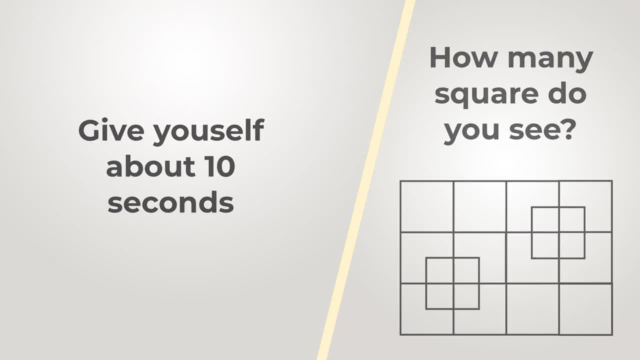 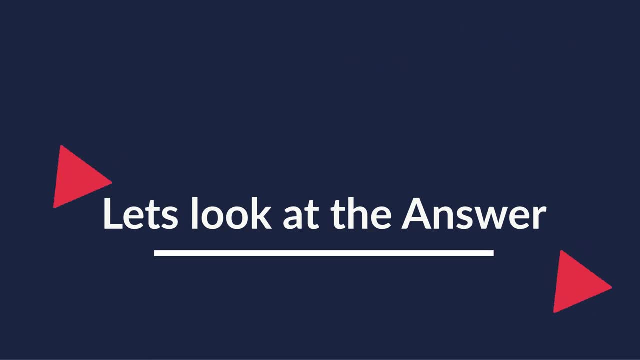 to find out the answer. feel free to pause this video if you need more time. do you have the answer? let's continue to see if we can come up with the solution together. as you might have figured out, there is a total of 30 squares shown in this picture. let's start by removing overlapping. 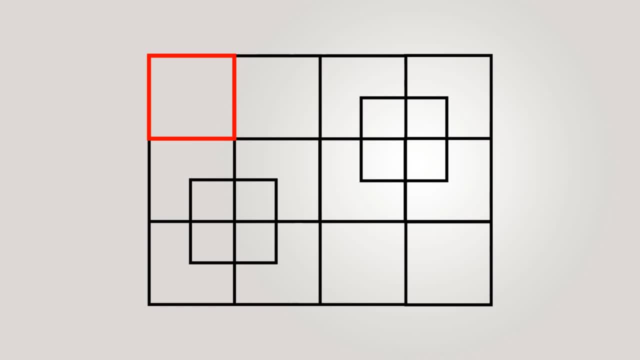 squares and counting medium-sized squares. there are 12 of them in this picture. let me count them all for you: one, two, three, four, five, six, seven, eight, nine, ten, eleven and twelve. once we reintroduce overlapping squares, we can count them as well. they would have numbers 13 and 14.. two overlapping squares introduce. 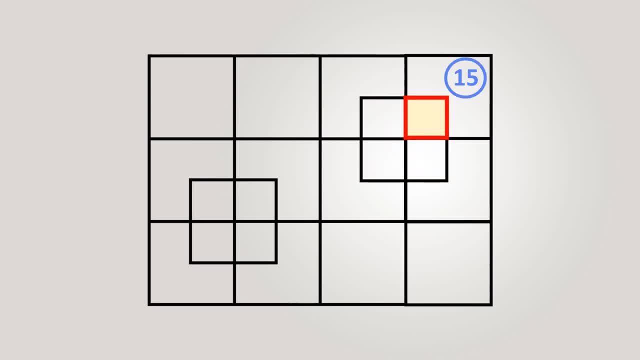 eight small squares. they would have numbers 15, 16, 17, 18, 18, 19, 20, 21 and 22.. there are also six large squares. let's give them a numbers: 23, 24, 25, 26, 27, and 28. 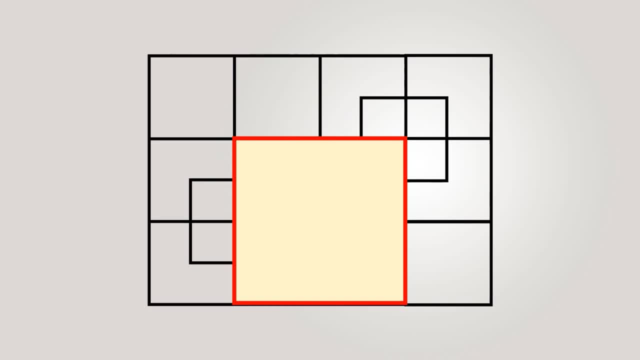 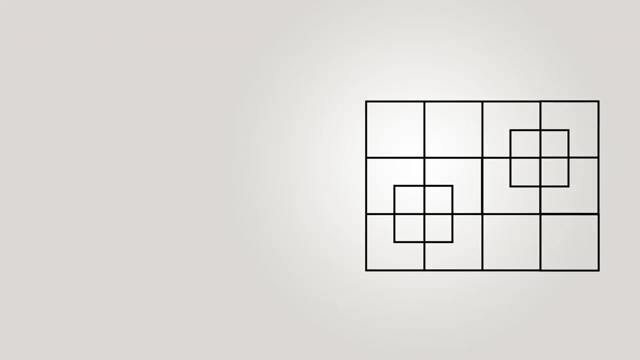 as you can see, those large squares are located in the top row as well as in the bottom row, and, last but not least, are two extra-large squares. I gave them the numbers 29 and 30.. Were you able to solve this challenge on your own? Did you get to the right answer? 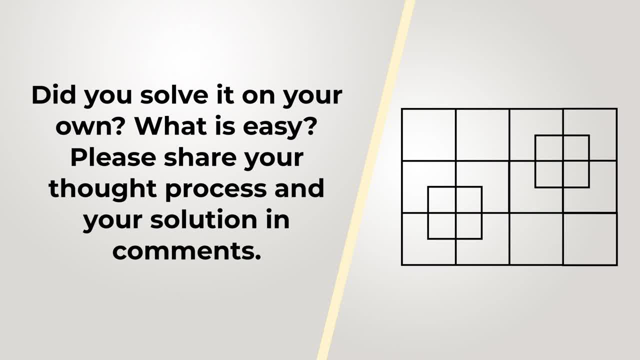 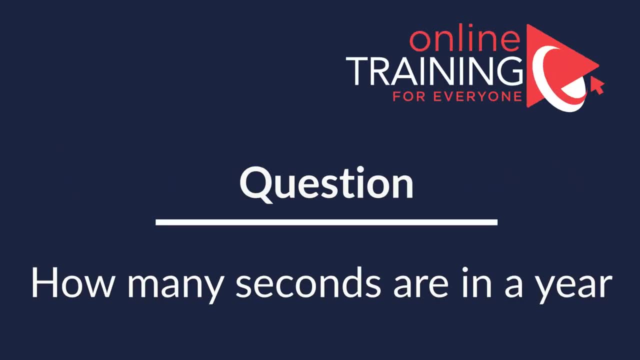 Or maybe we missed some of the squares. Feel free to share this information in comments and I hope this question was nailed by you and now you know how to answer similar questions on the test. I had this question being asked as part of consulting job interview. 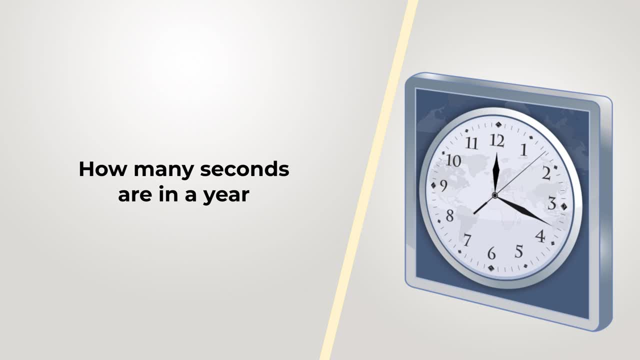 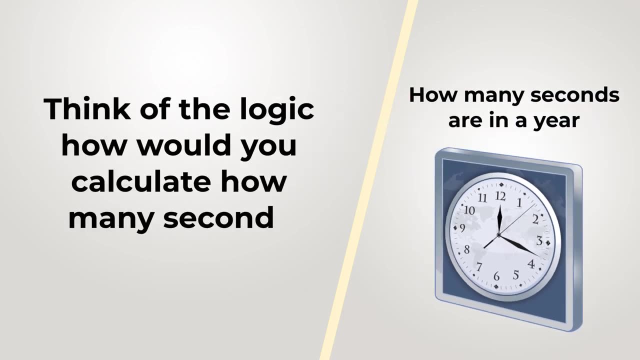 How many seconds are there in a year? Take a look at the picture. It might give you a hint. Do you think you know the answer? Think of the logic. how would you calculate how many seconds are there in the year? Or maybe there is an alternative. 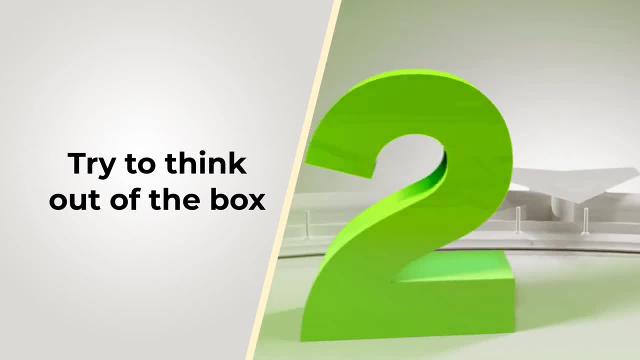 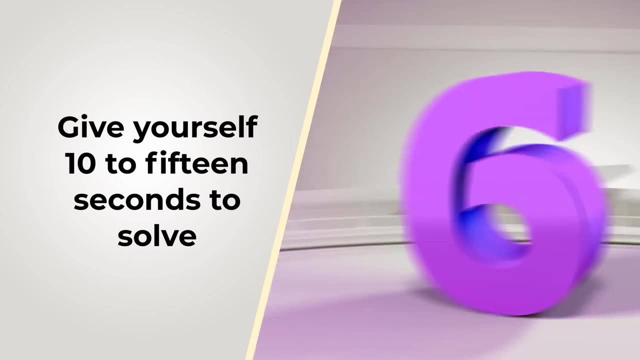 Always try to think out of the box- This would be my hint to you- And give yourself 10 to 15 seconds. This is as much time as you might get answering these types of questions in the test. Now let's continue and get to the correct solution together. 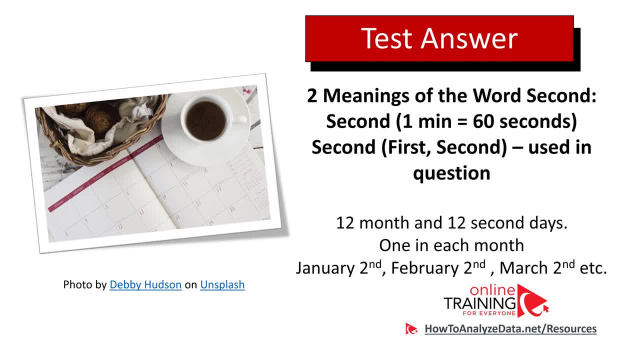 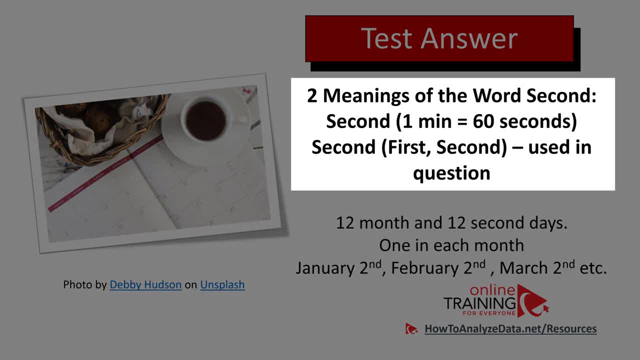 Obviously, this is a tricky question and it challenges you in understanding of the word second. There are two meanings in the word second. One is second- for example, one minute has 60 seconds, But the second one is second, where you have a sequence of four seconds. The second one is the second, for example, one minute has 60 seconds. Second is the second, for example, one minute has 60 seconds. But the second one is second, where you have a sequence of four seconds. 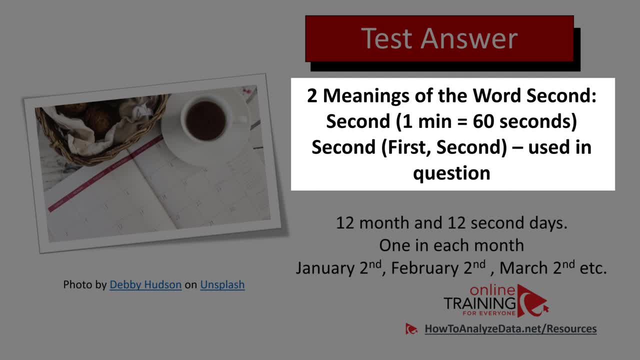 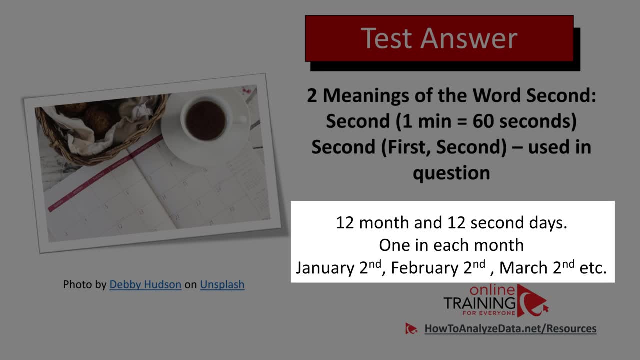 First and second, And the second meaning of the second is used in this particular question. So, if we go back to the question, In a year there are 12 months And there are 12 second days, One second day in each month: January 2nd, February 2nd, March 2nd and etc. 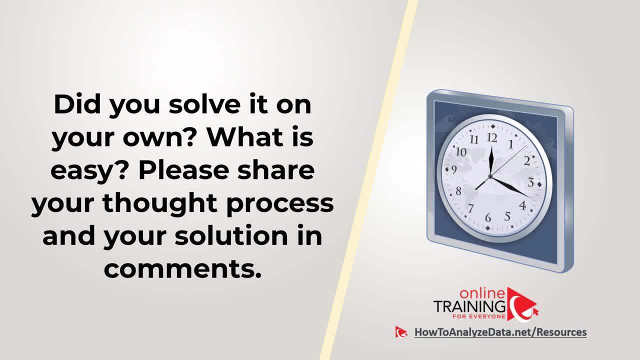 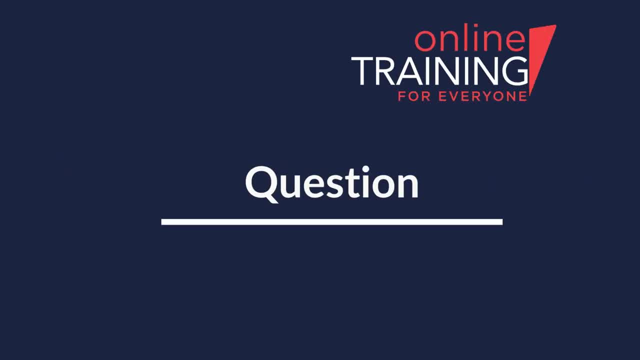 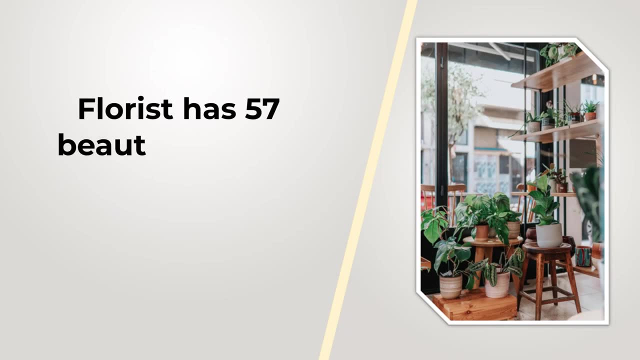 Hopefully you've nailed this question. It gives you some laugh And you now know how to answer similar problems in the test. Here is the challenging question you might frequently see on the test. Florist has 57 beautiful plants. All but 7 were sold. How many plants are left? 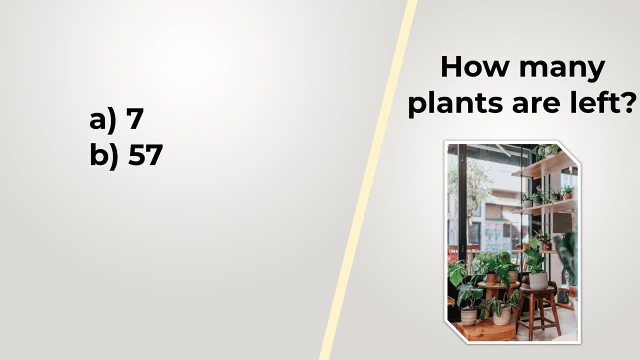 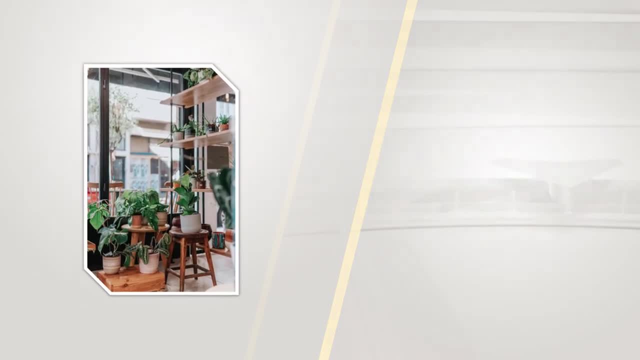 There are 4 different choices: 7,, choice B- 57,, choice C- 64, and choice D: 50.. Take a close look at this question and see if you might come up with the answer. Give yourself 10-15 seconds. 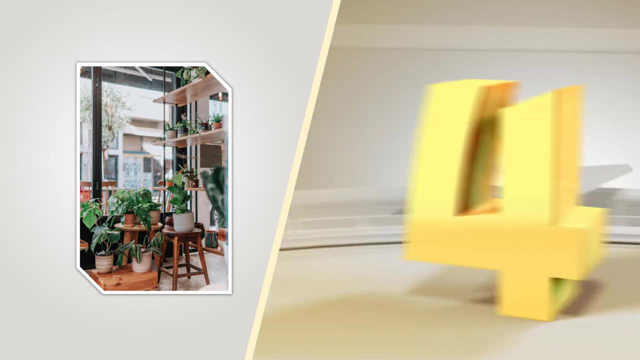 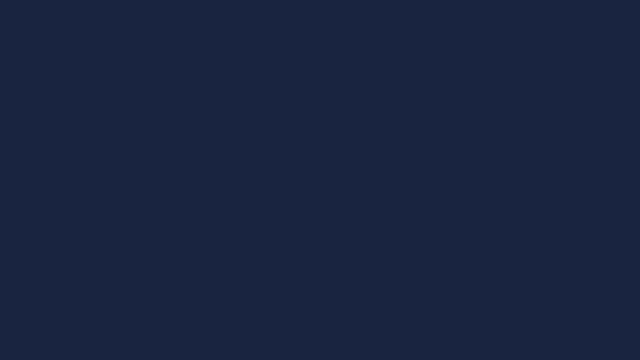 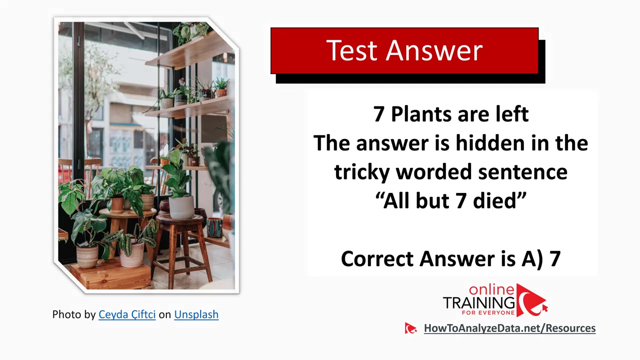 This is typically as much time as you would get on the test. Do you think you came up with the answer? Let's continue to see if we can solve this challenge and get to the correct solution together. I think you heard me correctly. So the answer is: 7 plants are left. How is it possible? 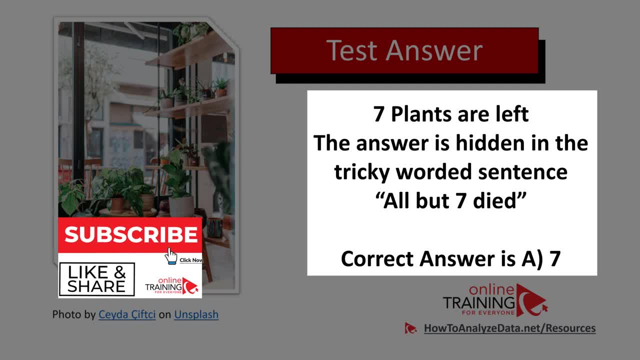 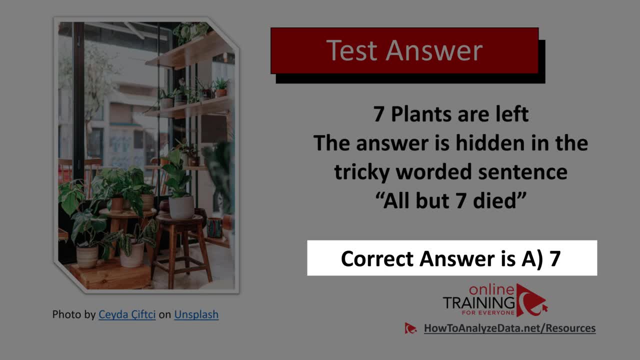 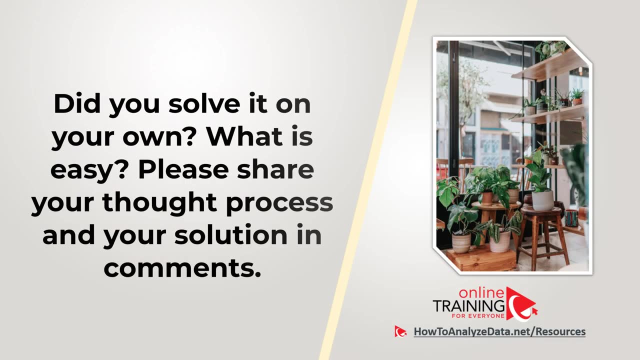 The answer is hidden in a tricky worded sentence: All but 7 died. So this is why the correct answer is A. Florist had 57 plants and all of them but 7 died. That's why the correct answer is A 7.. Hopefully you've nailed this question and now know how to answer similar. 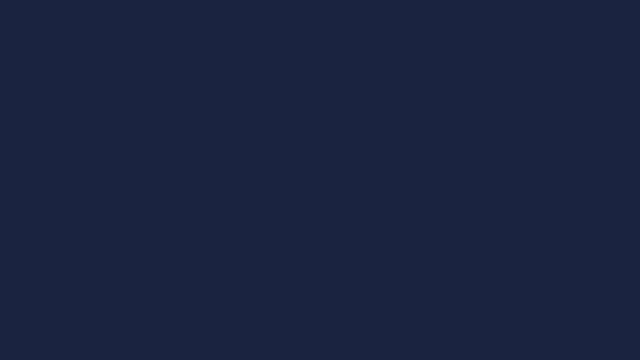 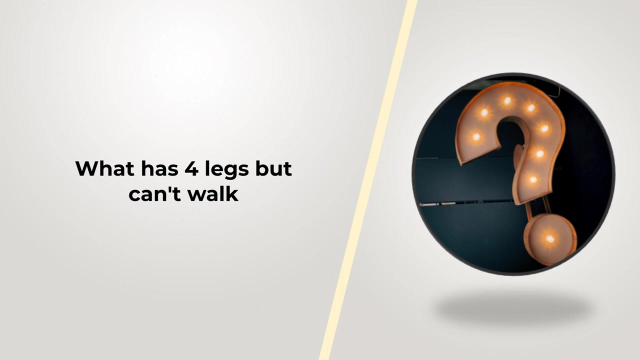 problems in the test. Here is the question which tests your understanding of English language, your vocabulary, as well as your ability in logical reasoning: What has 4 legs but can't walk? Do you think you know the answer? Now might be a good time to pause this video. 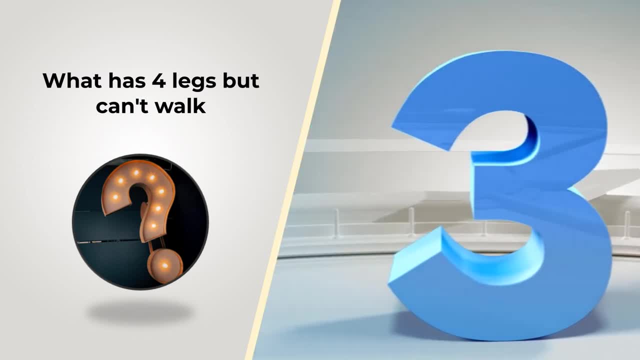 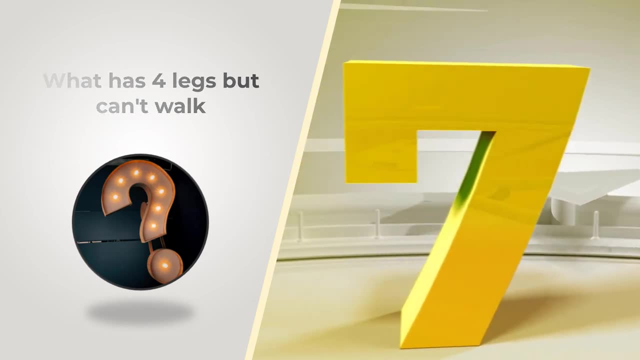 to see if you can come up with the answer. Do you think you found the answer? Let me give you a quick hint: Think out of the box and think of not necessarily something that walks. Did you figure it out? Let's continue to see how we can solve this challenge. 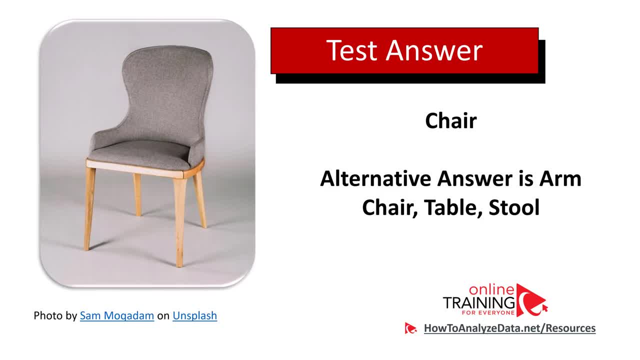 and get to the correct solution together: How to solve this challenge. As you might have figured it, the answer is chair And the alternative answer could be armchair, table or stool. As you might have figured it, the answer is chair And the alternative answer could be armchair, table or stool. 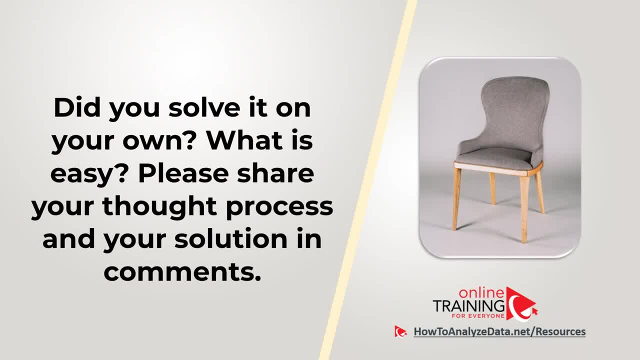 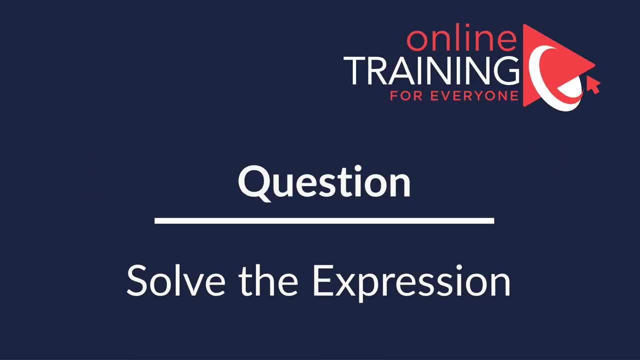 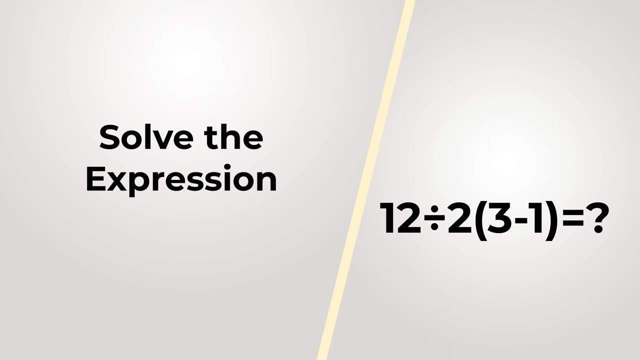 Hopefully you figured it out on your own and now know how to answer similar problems on the test. Here's the interesting question, which is easy to understand but at the same time, you will have a lot of fun solving it. You need to calculate the simple expression 12 divided by 2. 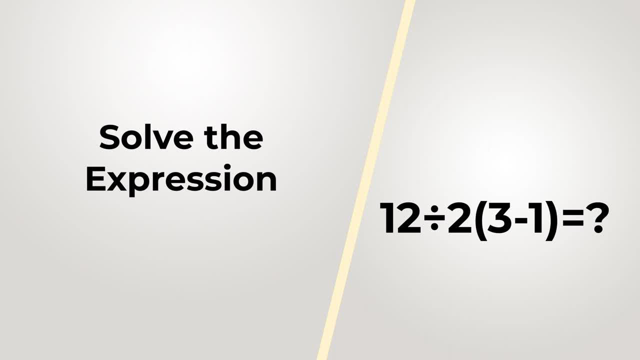 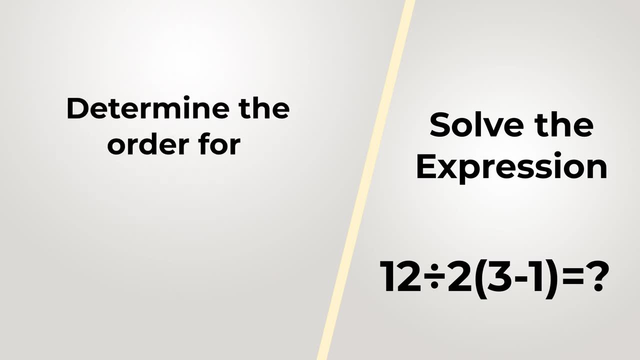 and then multiply it on the value in parentheses, which is 3 minus 1.. Take a look closely and see if you can come up with the answer. There are three operations here: division, multiplication and subtraction. All you need to determine is which one to do: first, second and third. 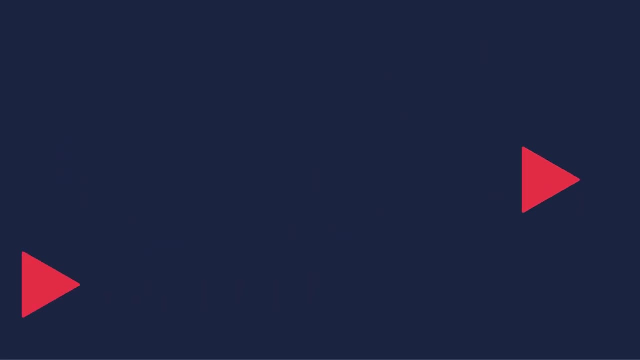 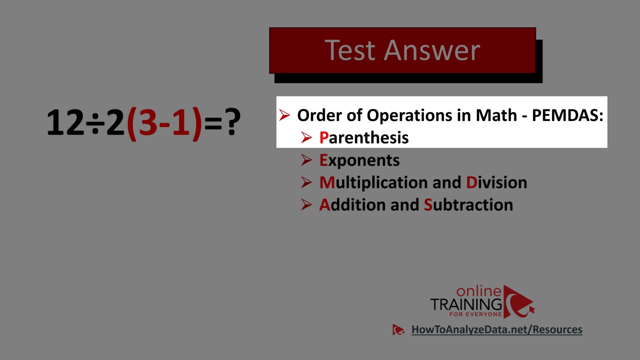 Do you think you know the answer? Let's continue and get it solved together. The order of operations in math tells us that the first expression we need to solve is in parentheses. We first need to calculate 3 minus 1.. An obvious answer is 3 minus 1.. 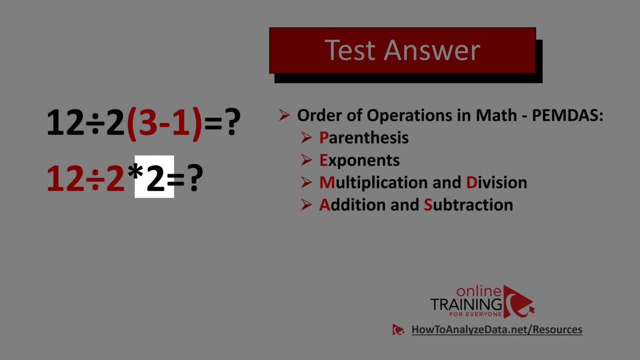 An obvious answer is 3 minus 1.. An obvious answer is 3 minus 1.. Obviously, the answer is 2.. The big question is: what do we do next? The order PEMDAS tells us that we need to do multiplication and division. 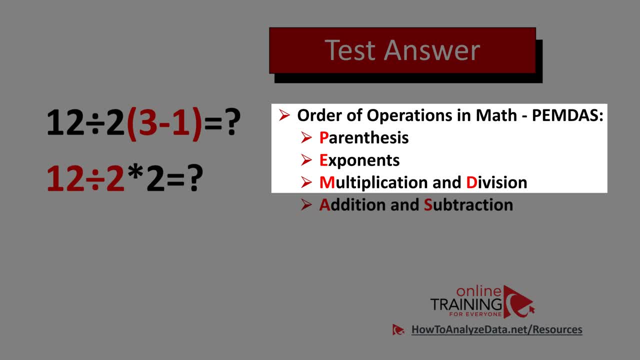 But what order doesn't mention is that we need to do it from left to right. And, what's interesting, the acronym itself is a little bit confusing because it shows multiplication first and then division. But in our case we need to do division first and divide 12 by 2 and then do multiplication Once we do. 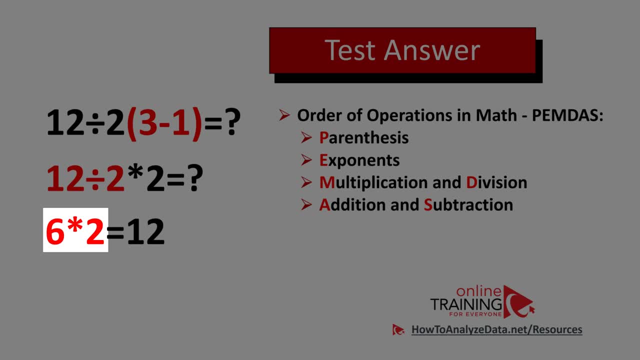 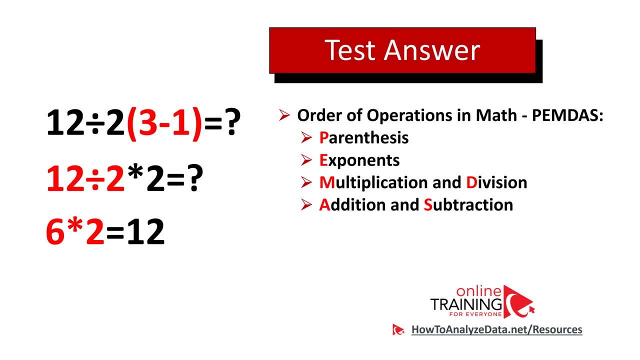 division first, and divide 12 by 2, we get to 6, and the final expression we need to solve would be 6 multiplied by 2.. So the correct answer here is 12.. Let me give you a quick hint, Even if you don't know the answer. 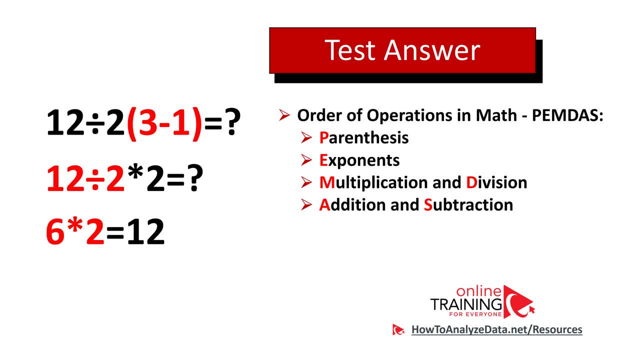 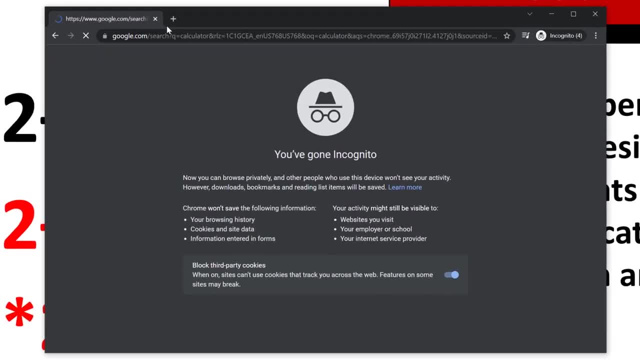 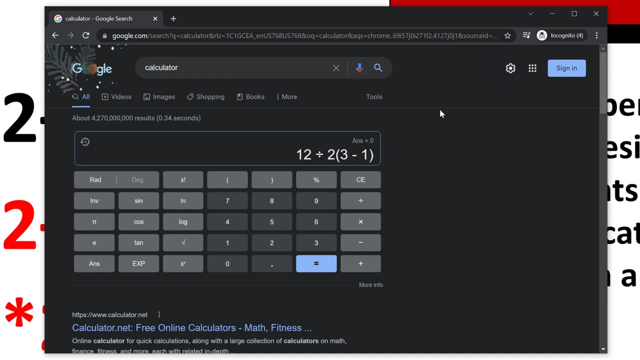 you can always use a calculator. Most modern calculators do support expressions. Let me demonstrate For example. if you type calculator in Google, it shows the calculator which you can use to solve the expression. You can preview the expression and once you hit the equal sign, 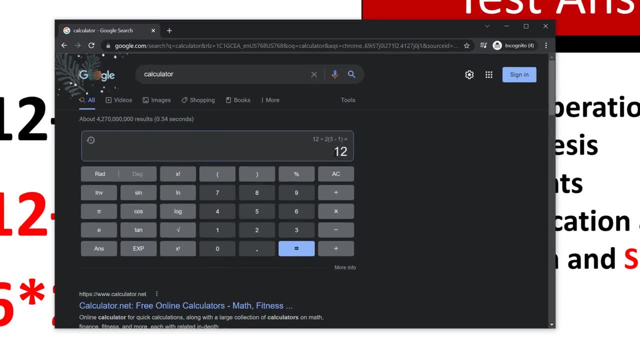 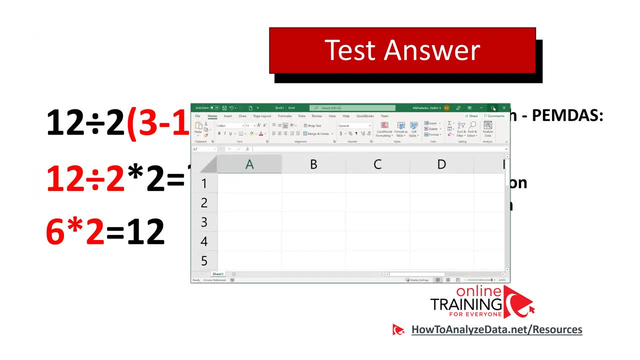 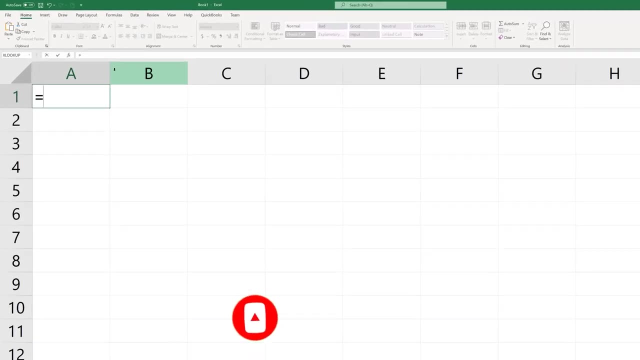 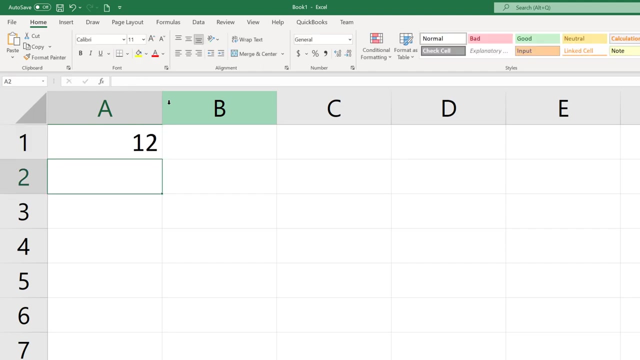 it calculates it for you And you can see that the correct answer here is 12.. Another alternative is to use Microsoft Excel, which is available on almost any Windows machine. Here you can enter the expression right inside any cell In Microsoft Excel. 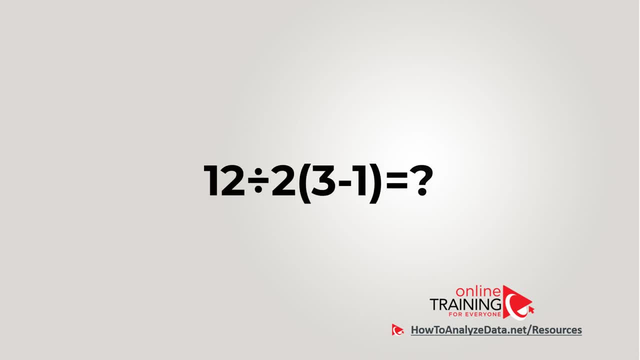 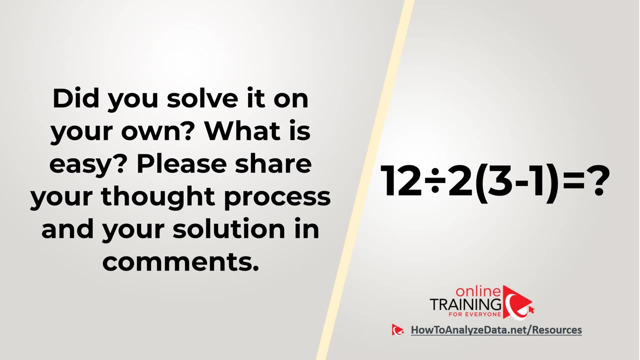 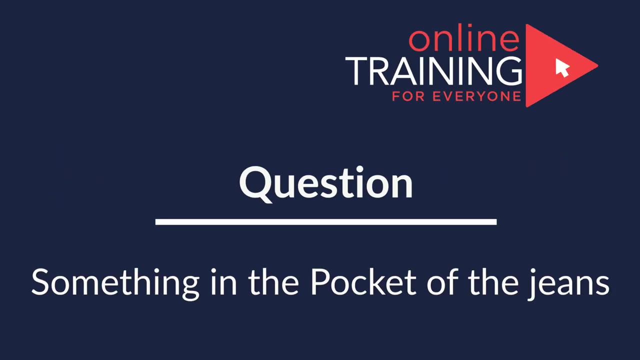 Microsoft Excel will perform the calculations. So did you solve this challenge on your own? Was it easy for you? Please share your thought process and your solution in the comments section of this video. Here's the interesting question you see sometimes on the test. It checks your knowledge of verbal. 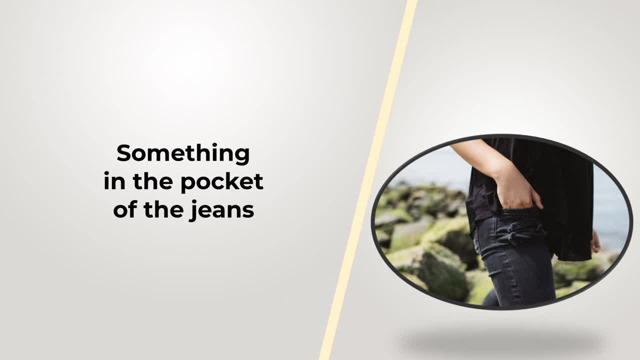 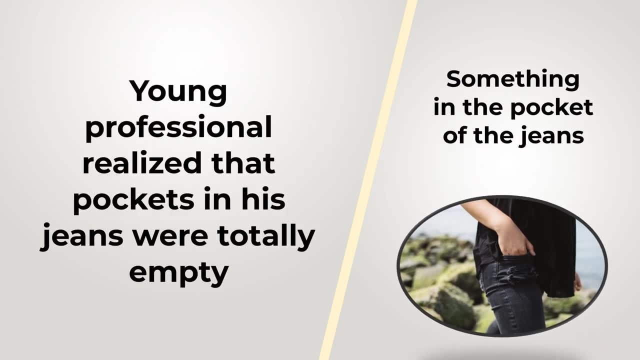 reasoning and understanding of the problem, And some people might argue that it tests your sense of humor as well. A young professional realized that pockets of his jeans were totally empty, But then he realized there was something else in there. How is it possible? 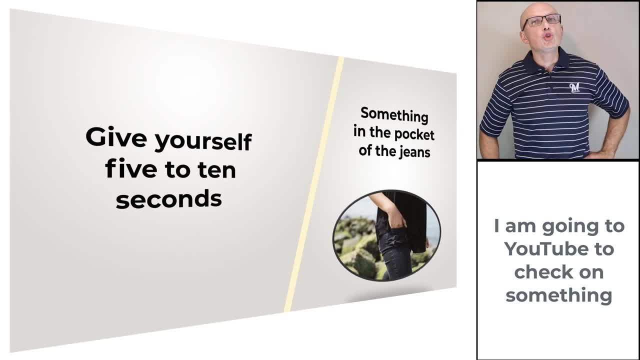 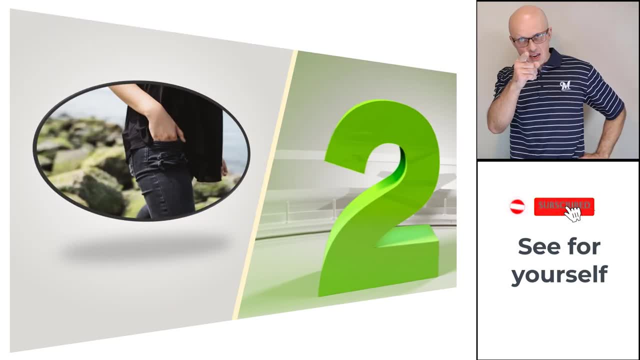 Do you think you know the answer? Give yourself 5 to 10 seconds, maybe 15 seconds. This is typically what you get on the test. Also, I'm gonna give you a hint: Please take a close look at the picture to see if you might see something unusual. 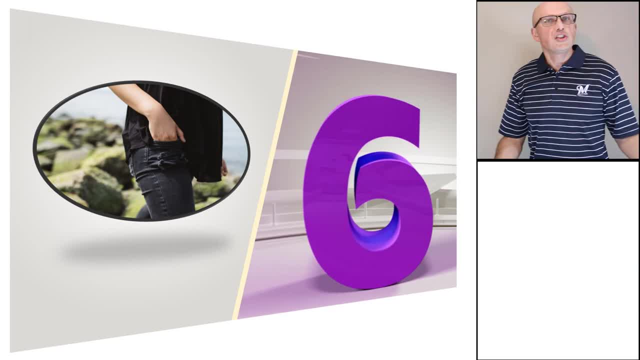 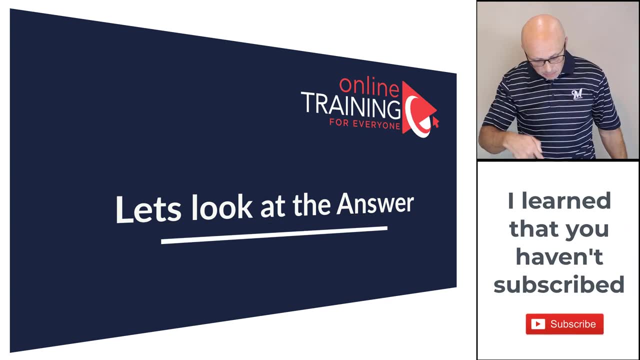 Do you think you know the answer? Let's continue to see how we can solve this challenge and get to the correct solution together. Let's continue to see how we can solve this challenge and get to the correct solution together. Do you think you know the answer? Let's continue to see how we can solve this challenge and get to the correct solution together. 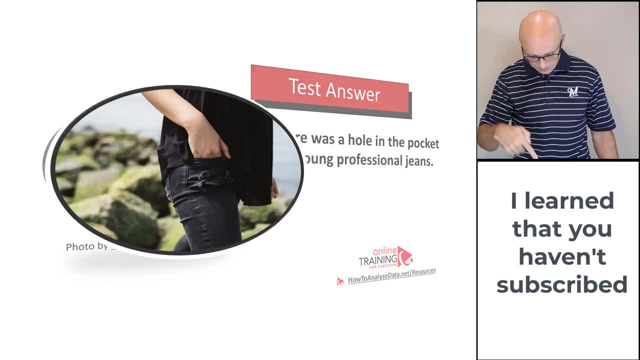 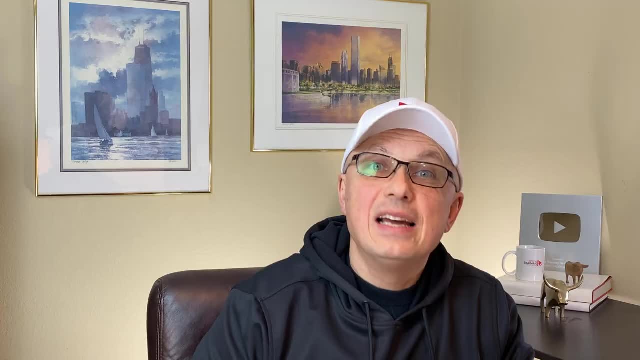 And the solution is very simple: There was a hole in the pocket of the young professional's jeans. Hopefully you've nailed this question and now know how to answer similar problems on the test. Thanks for watching. If you like the content, please give us a like and consider subscribing. 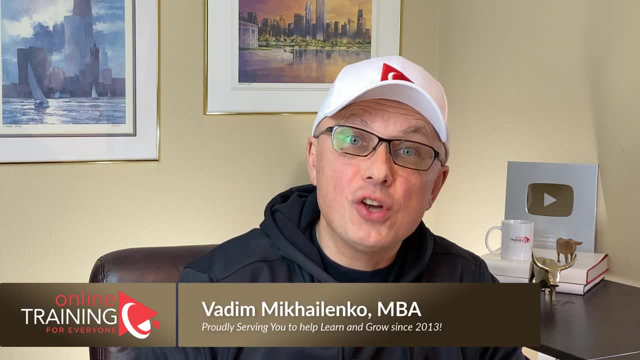 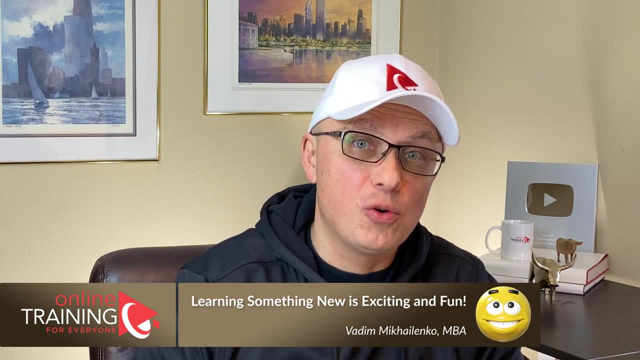 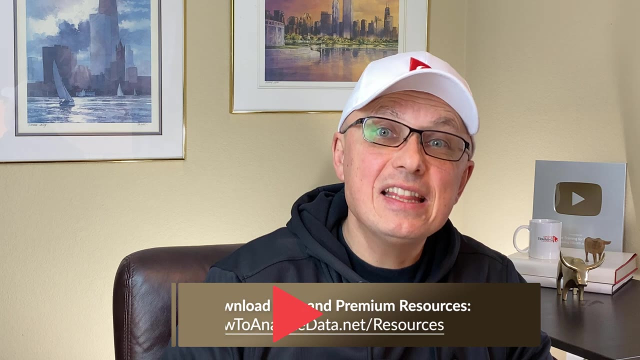 Thank you for your endorsement, support and patronage. Please also check out additional resources in the description section of this video. I also encourage you to check resources page on our website, howtoanalyzedatanet. Please leave your feedback, corrections or suggestions in the comment section of this video. 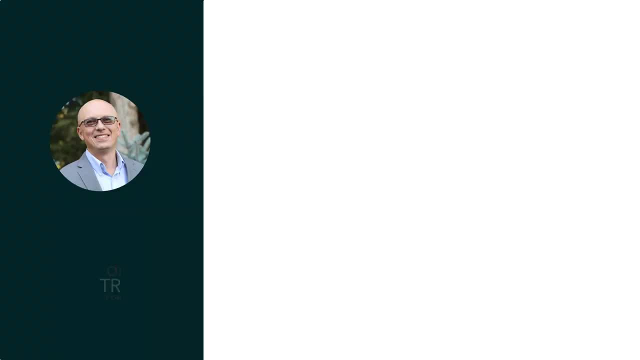 And all the best on your journey. I'll see you in my next video. Thank you for watching.